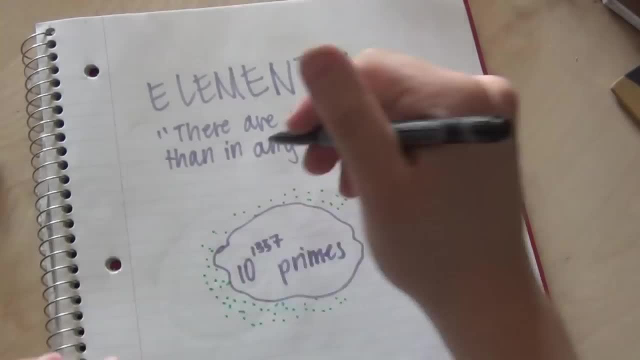 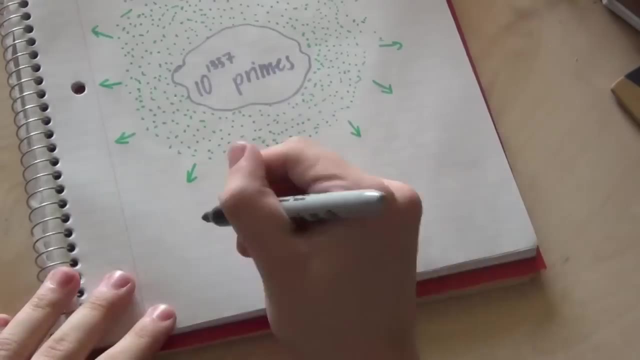 in any given collection, So in a collection of 10 to the 1357th power of primes, there are always more primes, Sort of like infinity, a proto-infinity To the Greeks and the Indians, the other mathematical center of the ancient world. infinity was not a conceivable concept, It was more of something. 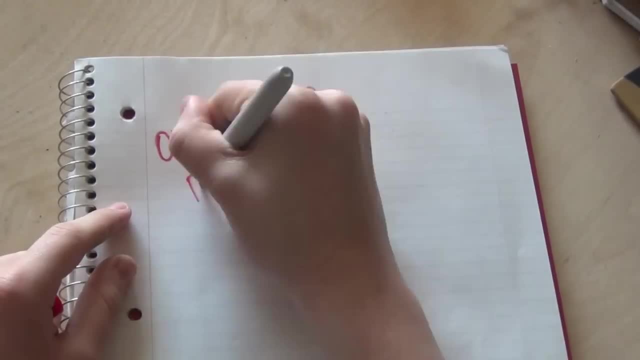 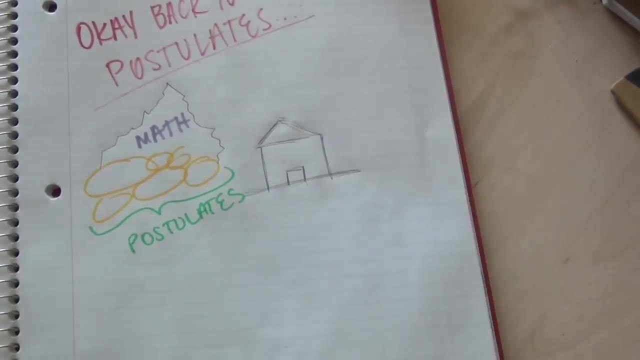 that you could approach using very fine philosophy. But let's not get distracted. Using postulates you can make a whole new set of mathematics. A set with a breadth of postulates is more stable than a set with only one foundational postulate, because if for some reason, one of the postulates 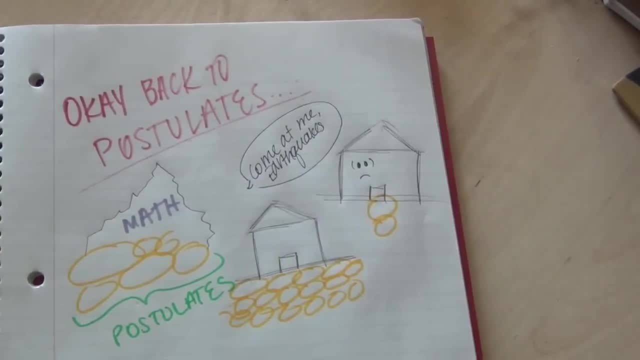 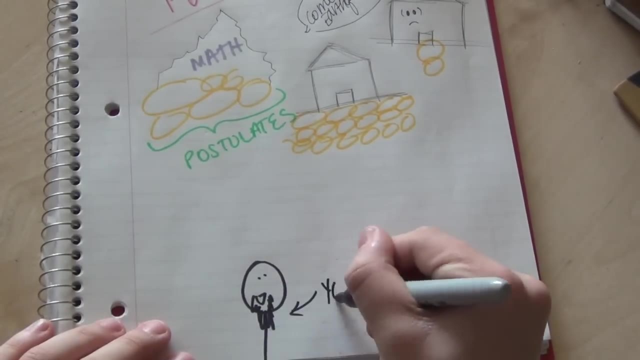 is proven wrong. then there are other postulates that maintain the integrity of the math you've created. But let's say that you're an ancient geometer and you don't know much about the history of mathematics, because, well, there isn't one. Let's actually say that you're 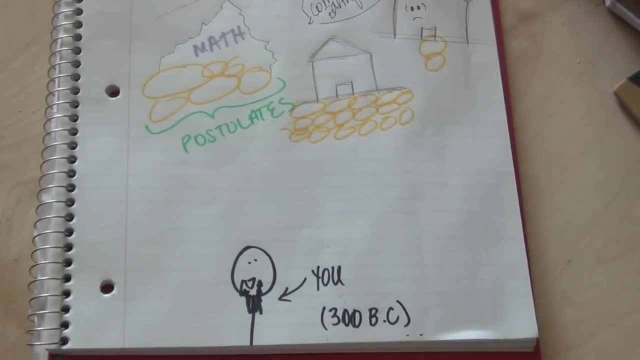 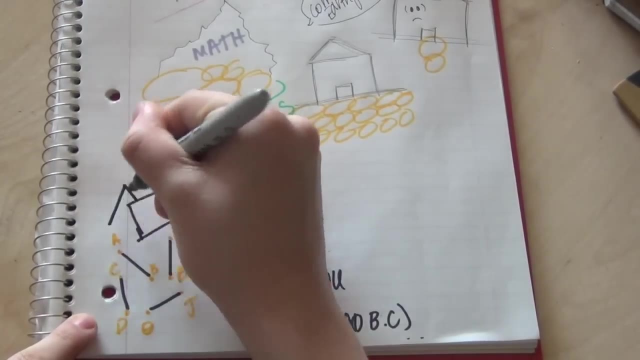 a Euclid and that you're sitting down to write the rules of geometry and you start writing out some of the self-evident postulates. Okay, so you'll be drawing a lot of line segments to show squares and stuff. so I guess that the first thing you say is that between 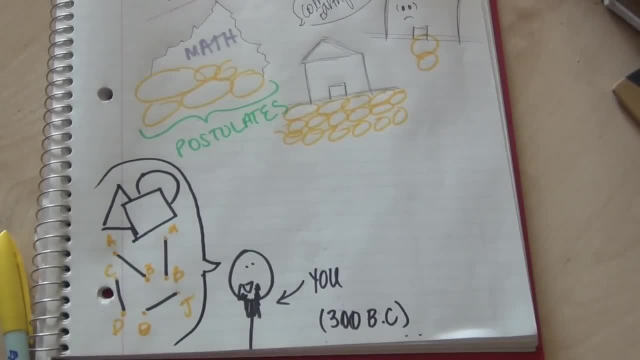 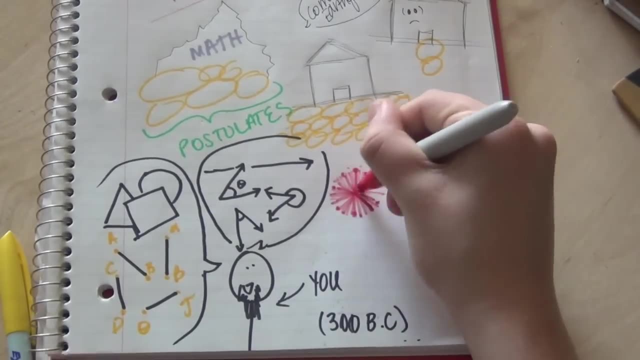 two points. you can draw a line segment. Now, you also know that angles extend forever if you don't get the battery, so you might as well call those indefinite segments lines. Oh, and also with any segment you can make a circle because, well, yeah, And all right. 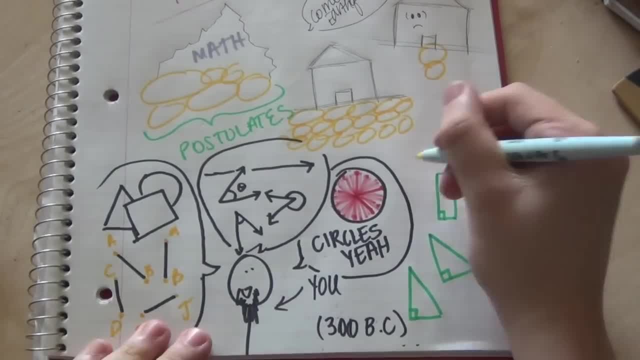 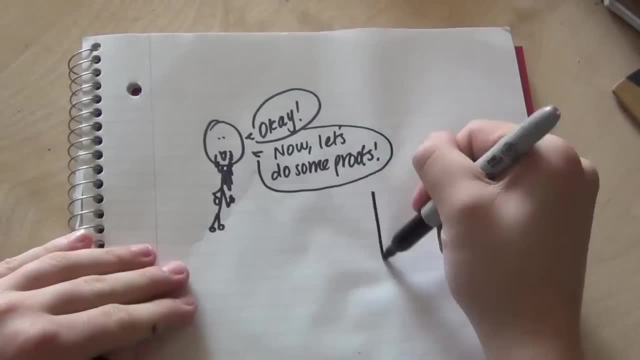 angles start congruent, because 90 equals 90,, whether you like it or not. you can draw a line segment And there you go. you've got the first four of Euclid's five postulates, But something doesn't seem right. You set up for these postulates and you try to start. 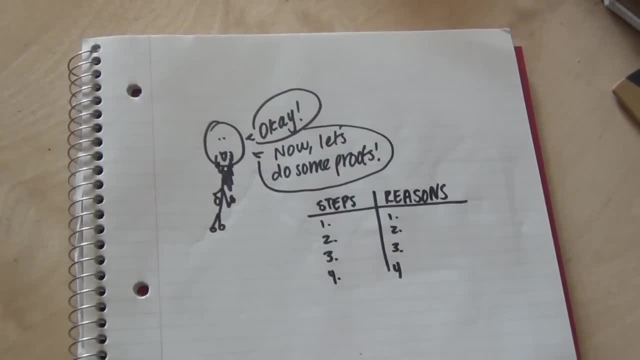 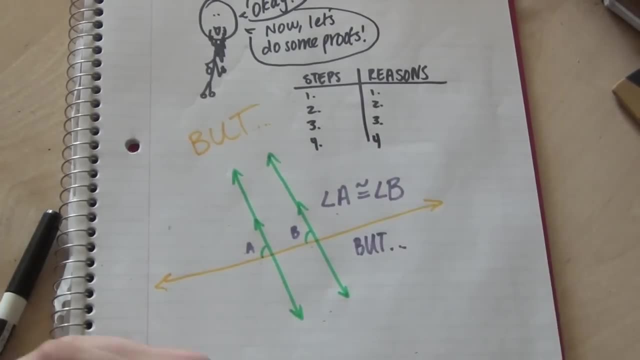 making proofs and at first everything is fine until you start using parallel lines. but wait a second. How do you know that the line you're drawing is the only parallel line when proving that when two parallel lines intersect another line, the resulting angles are congruent, Aren't there others? Well, no, This is called the parallel postulate. 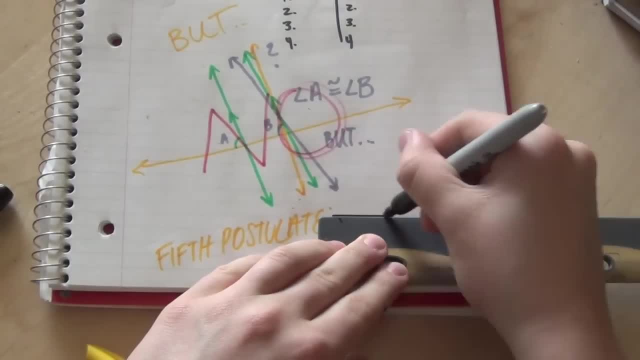 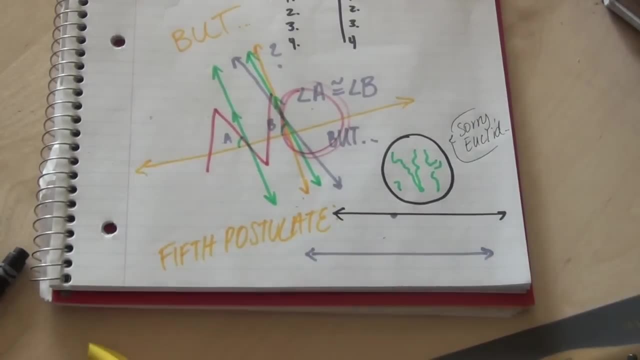 and it's Euclid's fifth and most controversial postulate. It states that if you have a line in a point that isn't on a line, then only one line that passes through. the point is parallel with the original and while that makes sense at first, it falls apart pretty. 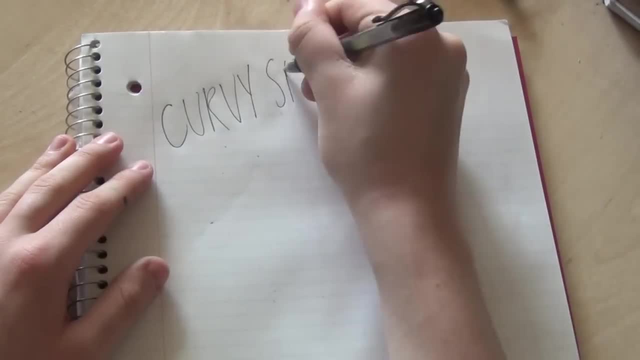 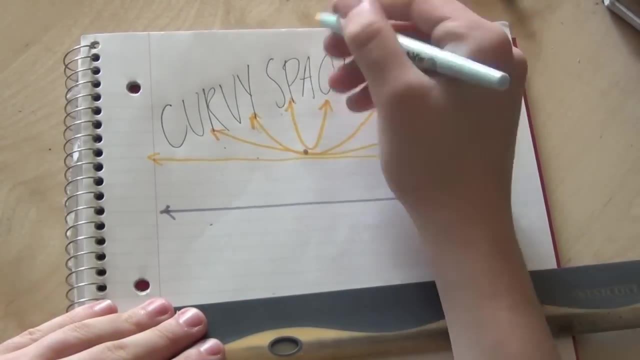 quickly when you realize that space actually curves and the Earth is a sphere. When you add the curvature of space into the equation, Euclidean geometry, which is based on the parallel postulate, falls apart, because you can have lines like parabolas and ellipses. 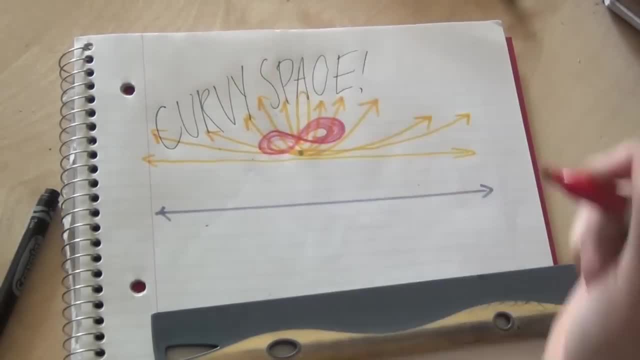 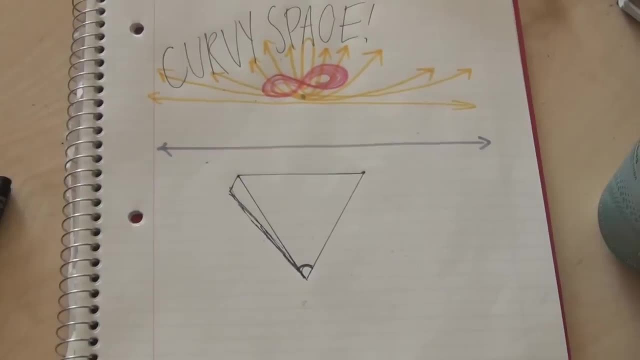 which I guess are just parabolas that collapse onto themselves, and you can come up with infinite different lines that pass through a point and are parallel, meaning they never touch the other line. You see, Euclidean geometry is like an inverted pyramid, and if you take away the tip, the 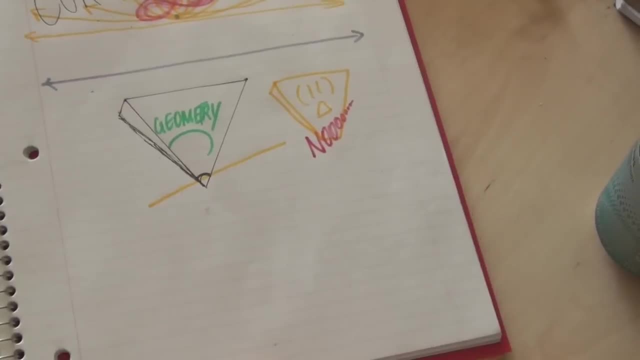 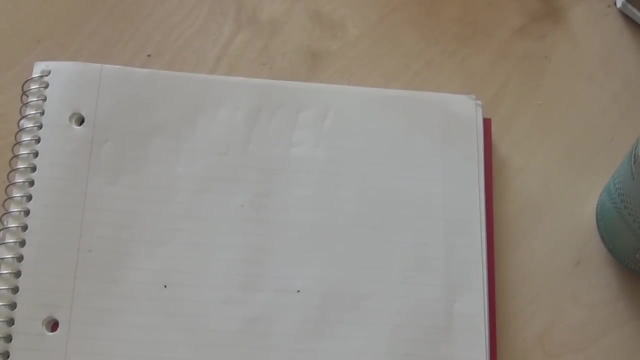 pyramid just crashes down onto itself. If there's no parallel postulate, then there's no Euclidean geometry. and then what? Can triangles' angles add up to more than 180?? Fah Well, actually yes, because on a spherical Earth you can move a triangular path and 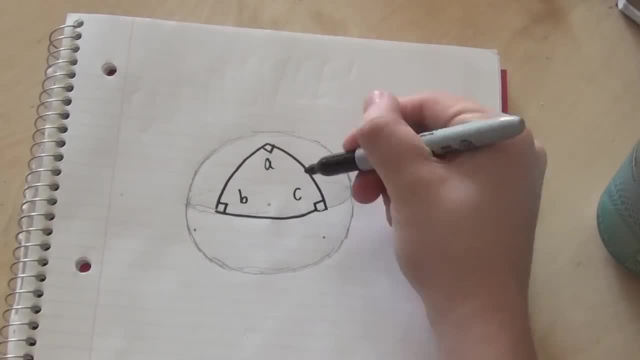 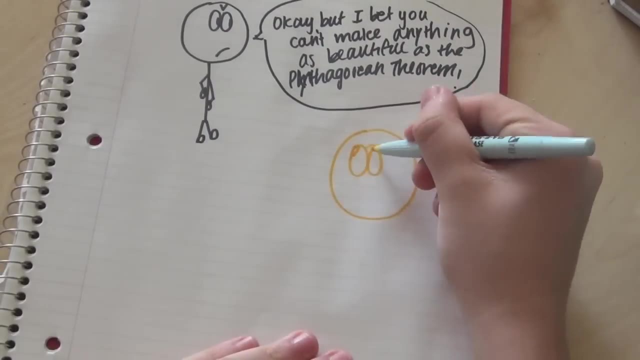 turn exactly 90 degrees each time, so you end up with a triangle that's 270 degrees. Okay, but I bet you can't make anything as beautiful as the Pythagorean theorem without Euclidean geometry. Except that you can, because the Pythagorean theorem was made like a hundred years before. 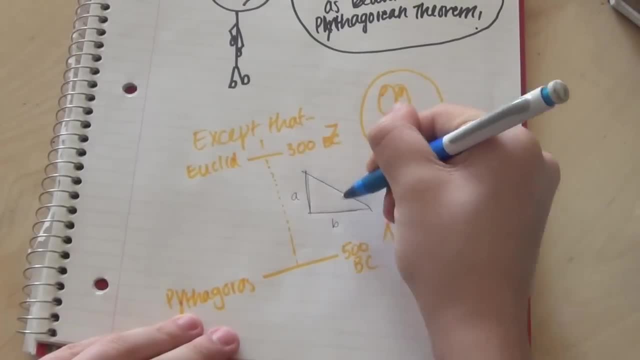 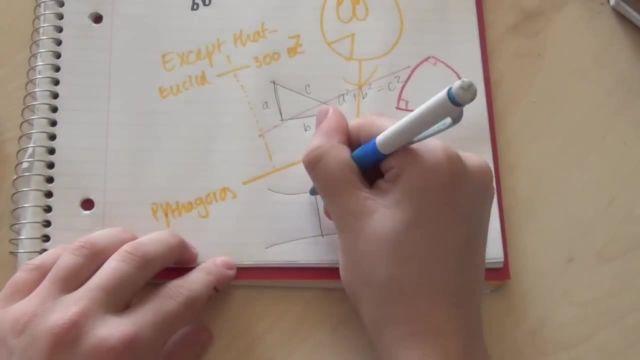 all this geometry stuff was even invented. Plus, the Pythagorean theorem doesn't actually work if your triangle's a right triangle but actually has three 90-degree angles. so ha, Without the parallel postulate you get all new sorts of geometry, like hyperbolic geometry. 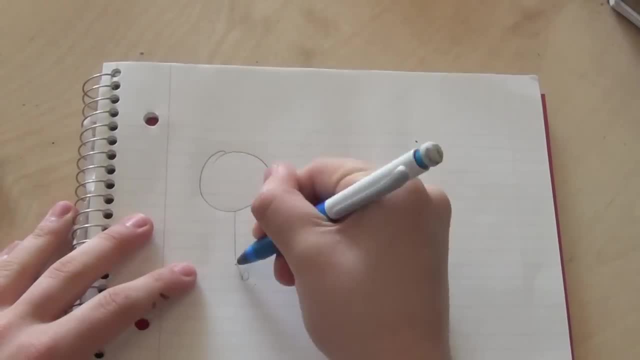 and elliptical geometry, where they're both just complicated ways of setting that lines curve, because space does too. All of this non-Euclidean stuff would make the Greeks cringe and it would probably make you look a bit unenthusiastic about life. since his 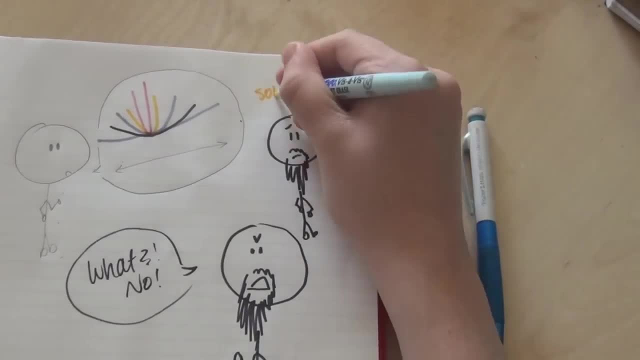 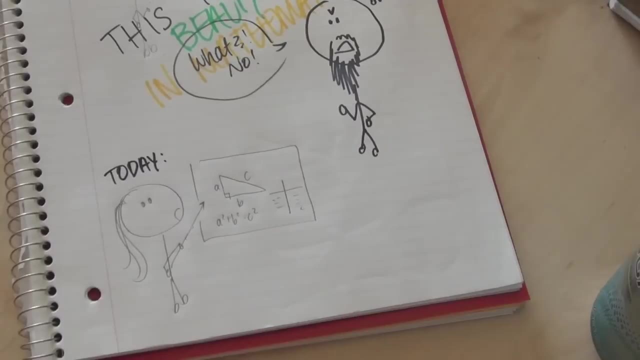 entire life's devotion was completely disproved. But when you think about it, it's not just the beauty in mathematics: Euclidean geometry is still not taught in school, Not because your administration thinks that your mind is too puny to understand the complexity of curvy lines, but because Euclidean 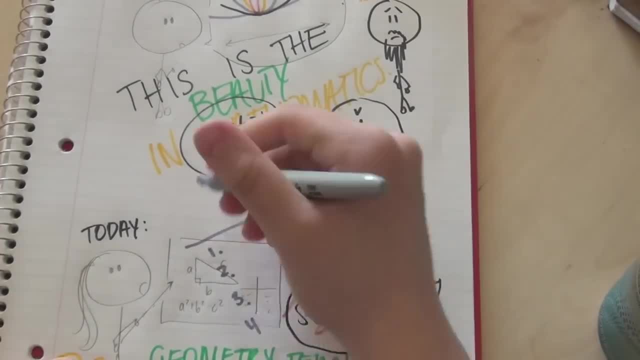 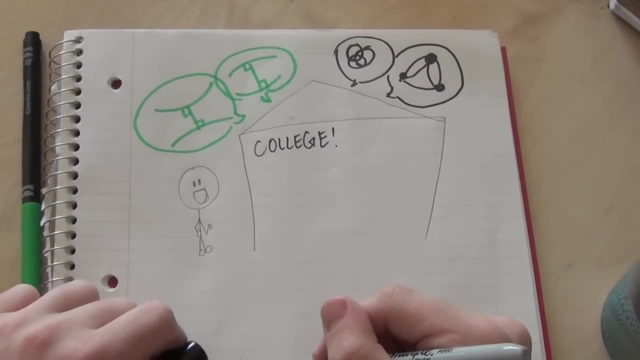 geometry still has real-world applications and because it teaches you real-world skills like deductive reasoning and learning to deal with mundane things like proofs. And you can still go to college and learn about hyperbolic and elliptical geometry or topology or graph theory, which is sort of contingent to geometry, and then you can 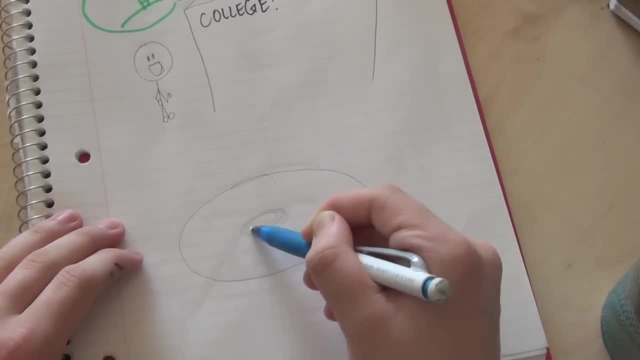 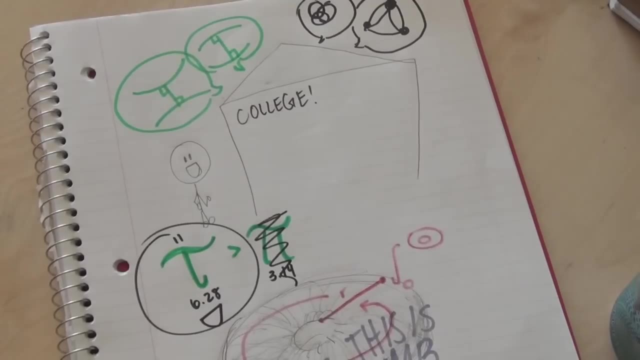 explain to your beloved math teacher Why trying to find the area of a torus while in Euclidean 9th grade geometry is a pointless endeavor, because in Euclidean geometry things like tori would be unrealistic and you should be focusing on the reasons why pi should be scrapped from the basic curriculum and you 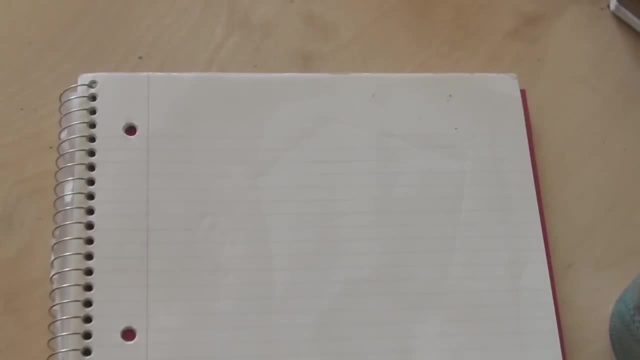 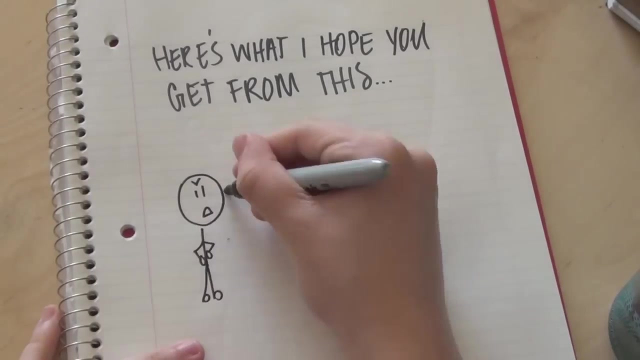 should use tau instead. Here's what I hope you get from this. While something super complex and weird like curvy space in which all the laws of geometry fall apart seems daunting and overwhelming, it can actually be cool and exciting, But that shouldn't distract you from appreciating the 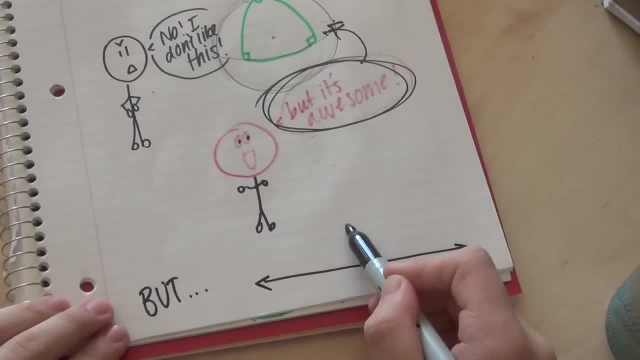 simple things like how to find the area of a torus while in Euclidean, 9th grade geometry, or how to find the area of a torus while in flat space. There really is only one line that goes through a point that's parallel to another.